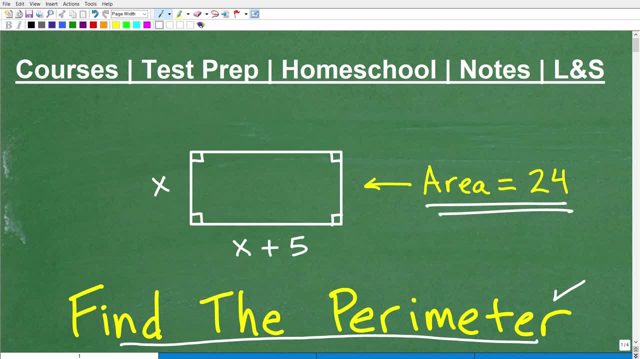 I'm going to give you a hint here. Matter of fact, you can probably see the hint in the title of this video. But anyways, let's just talk about this figure here real quick. Now, let's suppose I didn't tell you this is a rectangle. Could you interpret that in fact this is a rectangle, just based upon the figure? 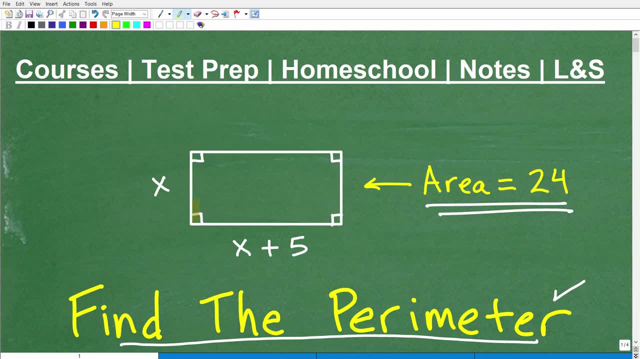 Well, hopefully you could. Let's just look at it. Well, you can't say that this thing looks like a rectangle, Therefore, in fact, it must be a rectangle. It never really works that way in geometry. But what you can confirm is that we have a four-sided polygon, ie a quadrilateral. for those of you who need to kind of review those terms, 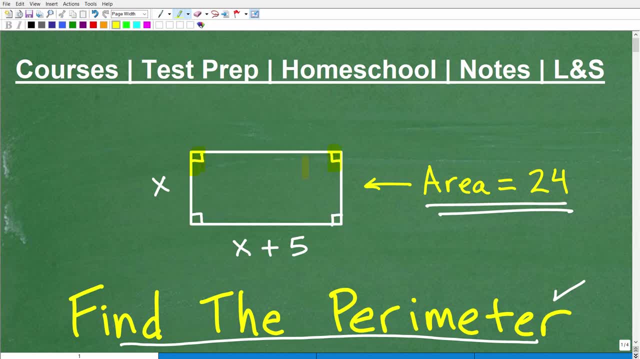 Or maybe you never heard those terms before, But these things right here, these little boxes in the corner, indicate that these are right angles, ie 90 degrees. So in fact, this is by definition a rectangle, which means that the opposite sides- this side here- is the same as this side, the congruent. 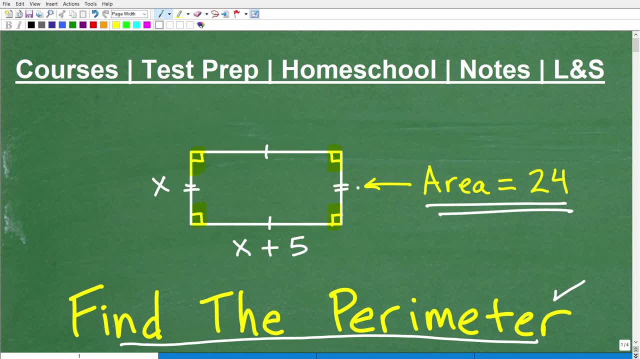 And then this side is the same as this side. So I'm going to give you some nice hints to be able to solve this problem, And in the title I give a hint. So if you're going to do this problem yourself, you're going to need to form a quadratic equation. 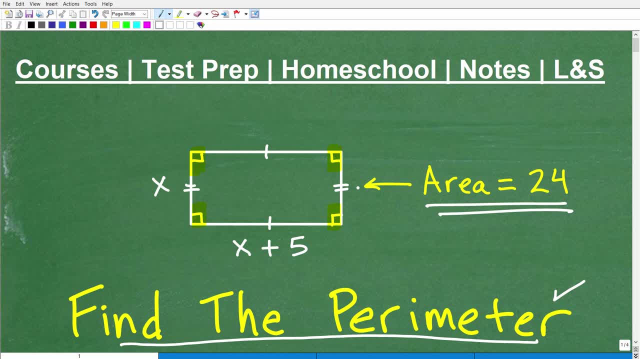 So this is a very typical, classic type of word problem that you'll see in any kind of algebra course: Algebra 1,, Algebra 2, etc. So if you want to go ahead and try to do this, go ahead and put your answers into the comment section. 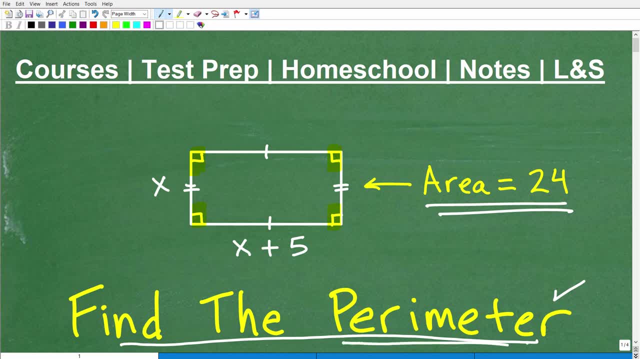 Again be very specific about what the question is asking when looking for the perimeter of this rectangle. So I'm kind of giving you extra hints here, But anyways, We're going to get into this in just one second. As a matter of fact, I'm going to show you the answer. 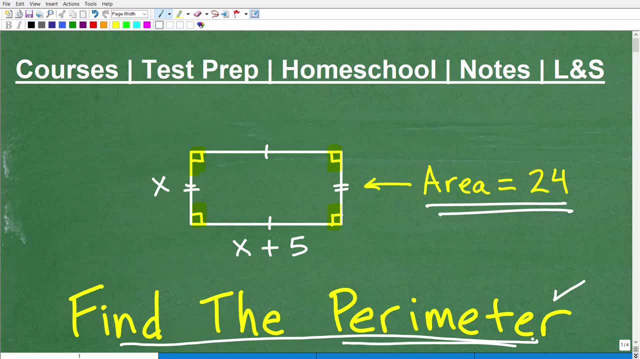 But first let me quickly introduce myself. My name is John. I'm the founder of TC Math Academy. I'm also a middle and high school math teacher. I've been teaching math for decades And I'm telling you right now: you can be successful in mathematics. 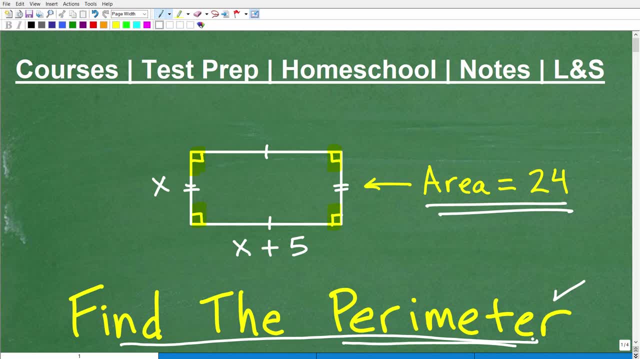 And I'm especially speaking to those of you out there that struggle in math. Maybe you don't like math, Maybe you think you're a bad math student. I'm telling you, don't believe that. What you need is great math instruction. 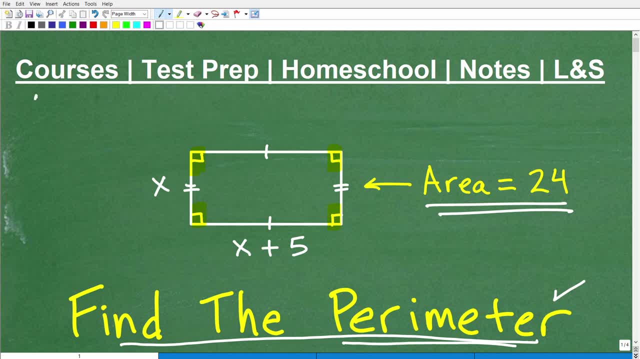 Clear, understandable and comprehensive. So if you're at the middle school, high school or even college level in terms of your math course, check out my math help program. I'm going to leave a link to it in the description of this video. 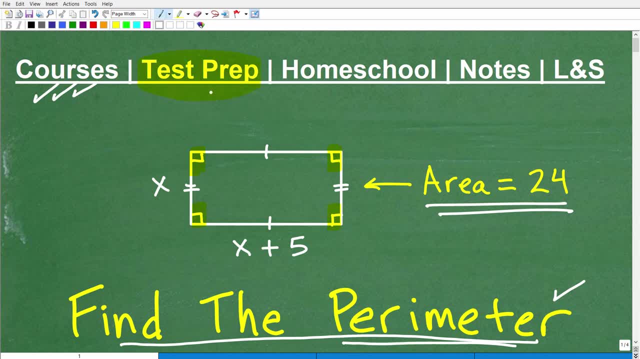 It will help you out big time, I promise. Also, if you happen to be preparing for a test with a dedicated math section, many of you are going to be taking a test like this. You don't even realize it. I'm talking about entrance exams, placement exams, certification exams. 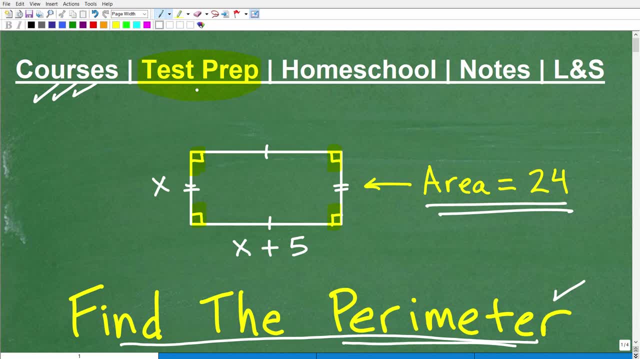 things like the SAT, ACT, maybe the ALEKS, ACCUPLACER, GRE, GMAT, ASVAB, TPS, etc. Anyways, I have a ton of test prep courses that can help you prepare and pass those exams. 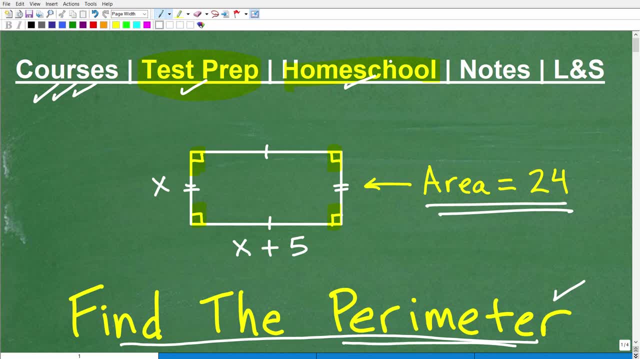 If you homeschool. I have award-winning middle and high school math courses for homeschoolers. There's a whole homeschool program, so check that out if you homeschool. If you need great math notes, I'm going to leave links to my notes in the description of this video. 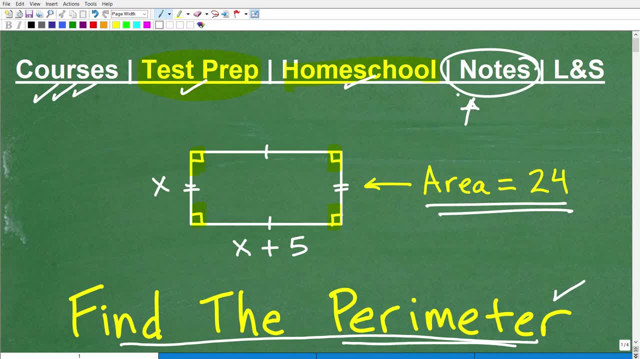 Hopefully you have your own great notes. If you do not, you need to work on note-taking, as this is critical to be successful in math. If this video helps you out, don't forget to like and subscribe, as that helps me out. 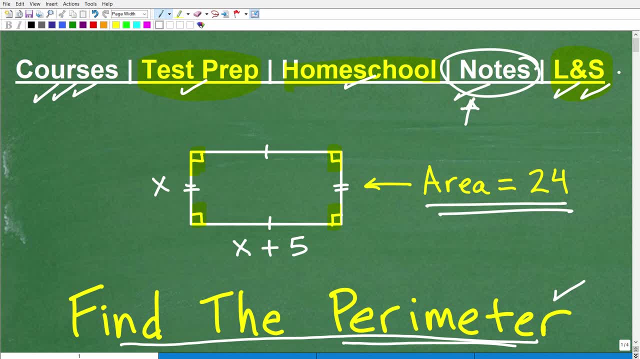 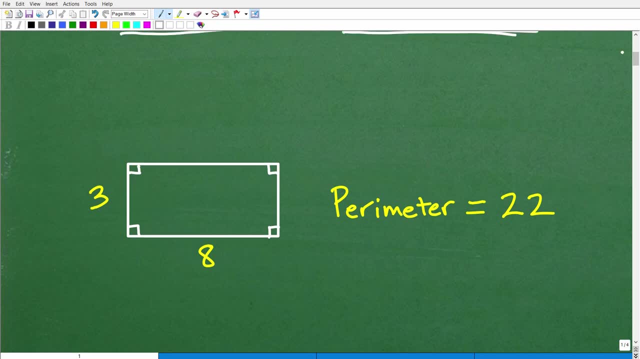 I'm going to show you the answer right now. If you don't want to see it, pause the video Again. you are going to need a quadratic equation. It's a bit of a hint. Here is the answer: The perimeter is 22.. 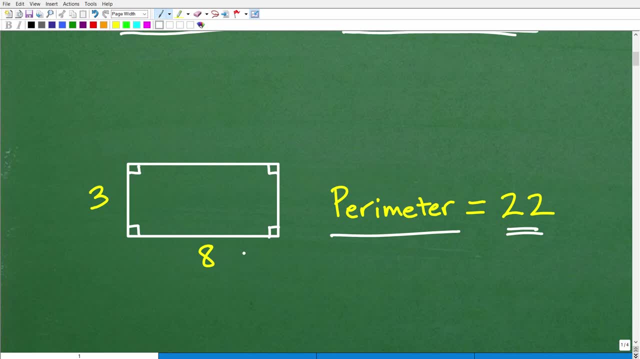 This would be the dimensions of this rectangle. If you got this right, I must reward you with a nice, happy face. an A++, a 100.. You know these days back in the good old days when I went to school in the 70s and 80s. 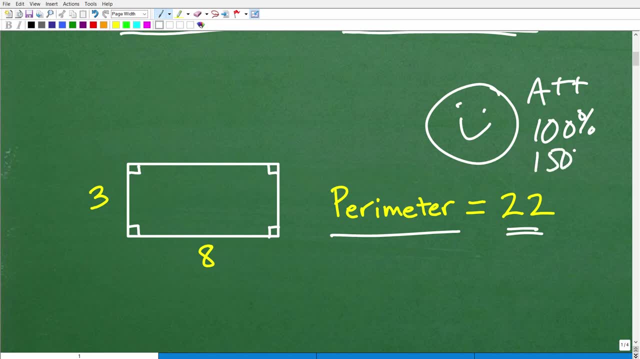 the best you can really do is 100%, But now you can go like 150%. Matter of fact, the GPAs- the best you could do. back in my days the GPA was 4.0. But now you can get like a 10.6 GPA. whatever the case is. 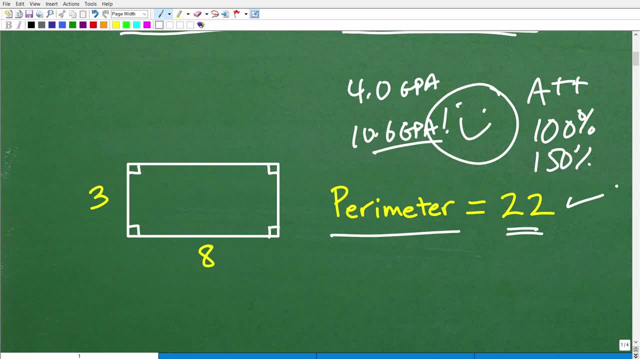 Listen, that's pretty awesome If you got this correct, nice job, Okay. so here's the thing I bet you, a lot of you put in 3 as your answer. Okay, What you did was solve this quadratic equation and you said, oh, I got the answer. 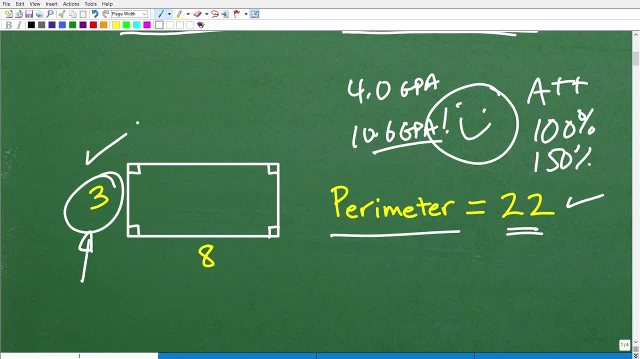 and maybe you just put in the result of solving that equation. That's a pretty common mistake. Remember that you need to always ask yourself: did I answer the question? And the question is: is not what the dimensions of this rectangle is? is what is the perimeter? 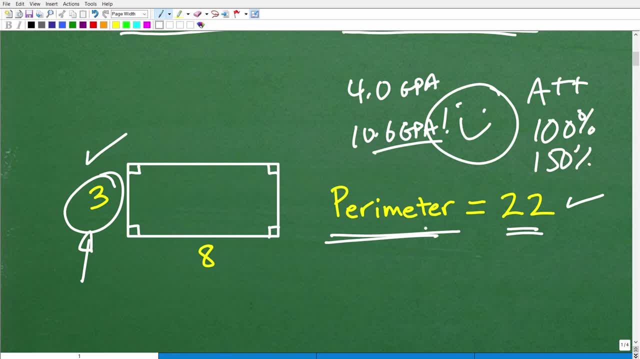 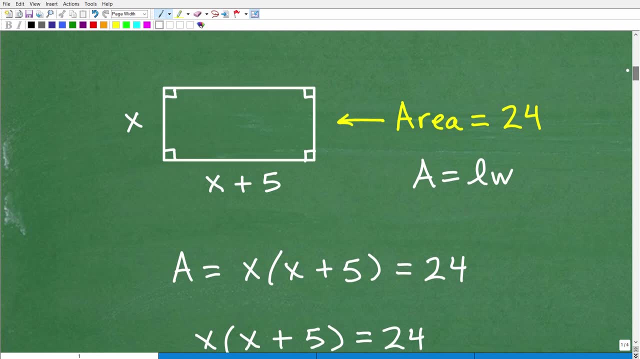 So we need to know what the perimeter is and how to calculate it. So I'm going to cover all this in just one second, But let's go ahead And take a look at what we need to do. Okay, So again we're dealing with a rectangle and we have a big clue here that the area is equal to 24.. 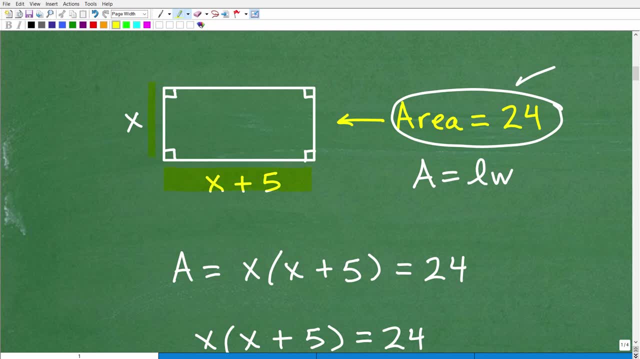 And we have the dimensions. This side here is x and this side is x plus 5.. So you're going to have to, we're going to have to involve this given information, this area and this figure to figure this thing out. 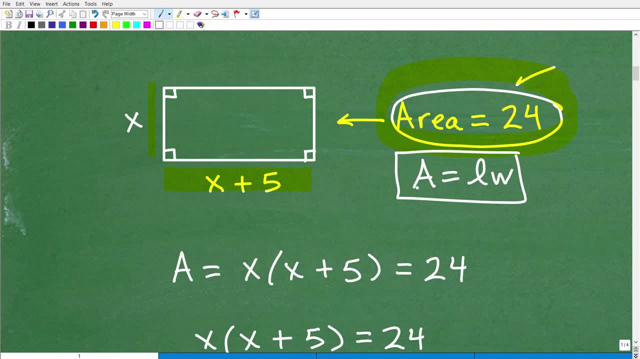 So, in order to do that, you need to know the formula for the area of a rectangle, and that's length times 1.. So length times width, and hopefully you already knew that. If you don't know that, this is one of these basic math geometry formulas that you should commit to your long-term memory. 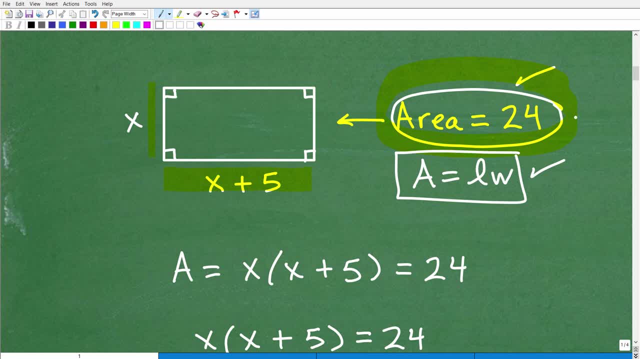 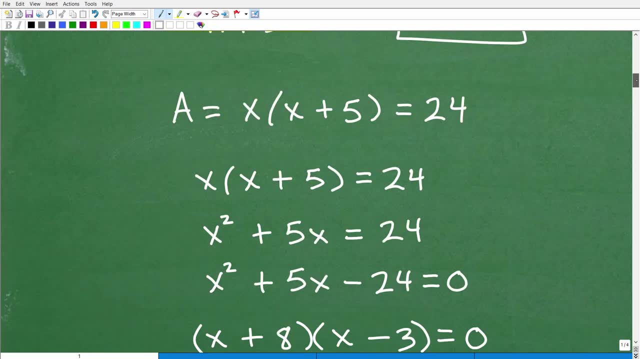 But anyways, the area of a rectangle is equal to length times width. So we're going to use this, this piece of information and this figure, to tie this all in, to write a nice algebraic equation. Okay, So length times the width. 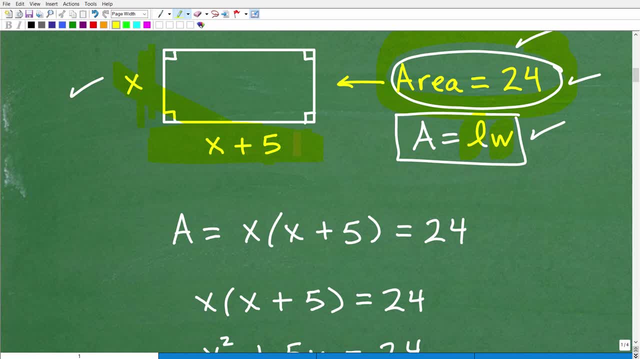 So here's the length, Here's the width. So we can just multiply this times this, And we know that this would be the area. So this side times this side, or the length times the width, is equal to 24.. 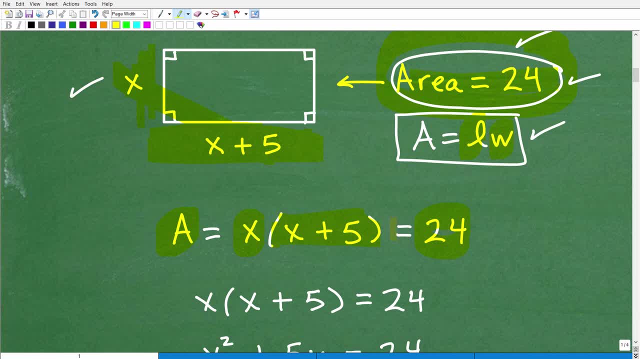 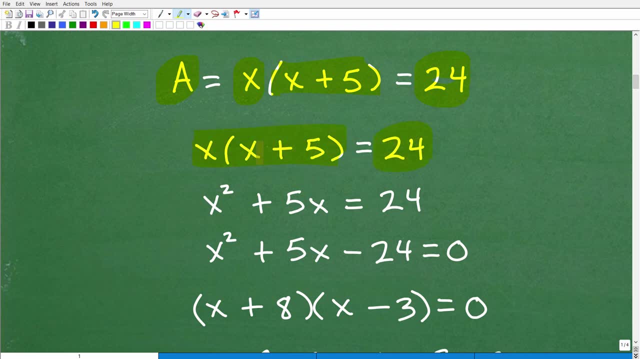 Okay. Or the area? Okay, Of course, the area is 24.. So basically, we have a nice equation here, All right. So x times x plus 5 is equal to 24.. This is, ie, the area of a rectangle length times width. 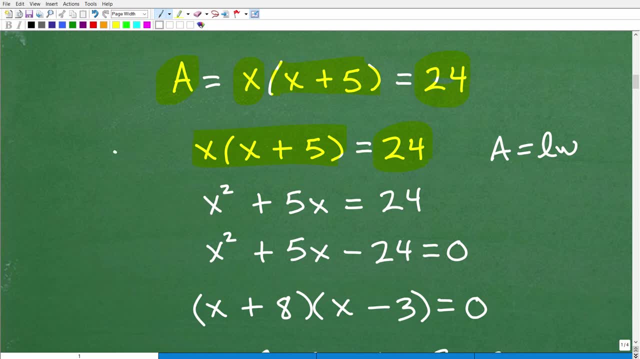 So we need to solve for x. So how do we solve for x? And this was the hint I gave you: that this is a quadratic. This is a quadratic equation. Now, what's the one thing we know about quadratic equations? 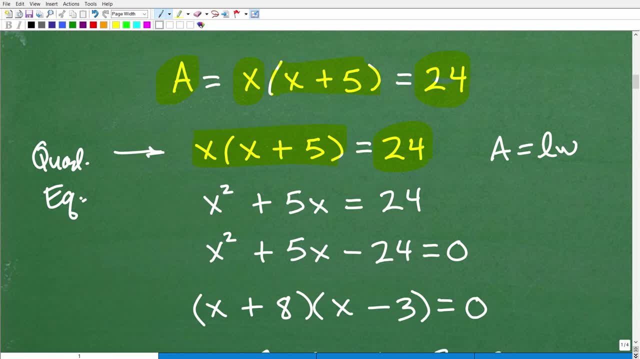 Well, hopefully you know a lot about how to solve them. If you do not, you know? I would say that you really, really need to review this, as this is critical. in terms of algebra, Okay, You absolutely need to know how to handle quadratic equations. 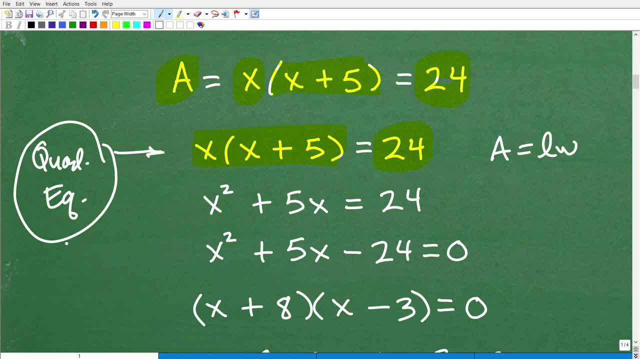 And this involves a good amount of skills. So there's different approaches. This particular problem works out pretty nicely, But you need to really make sure you understand quadratic equations. But the main thing here: Uh, Every quadratic equation is going to have two solutions. 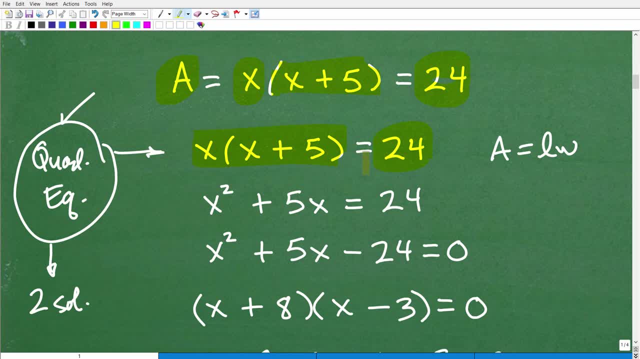 Okay, So we'll talk about that in a second, But let's go ahead and take our first step here. So we have: x times x plus 5 equals 24.. So what do we need to do? Well, right here, the way this particular format is, it's best that we go ahead and distribute this x into x plus 5.. 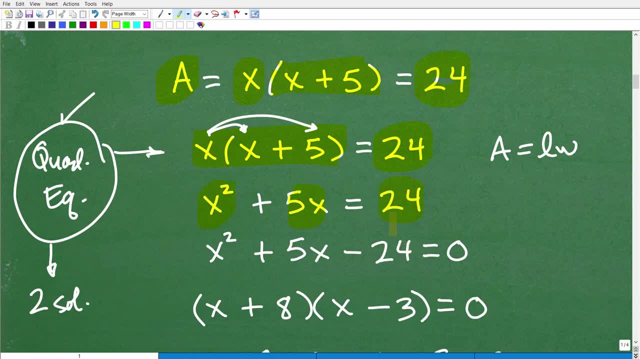 So we're going to end up with: x squared plus 5x is equal to 24.. So in a situation like this, We want to set this equation equal to 0.. So I need to subtract 24 from both sides of the equation. 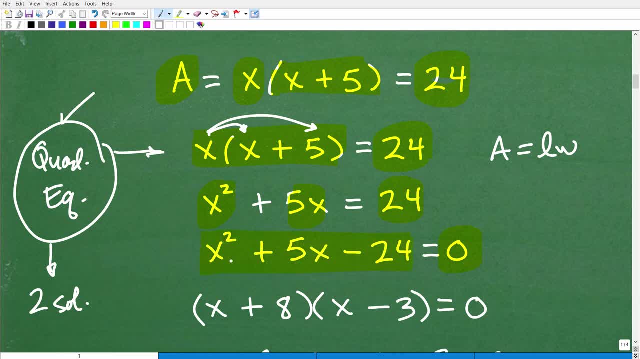 And this is what you have, Okay, So this is called a quadratic equation in standard form: Highest to lowest power. And then, here you may be familiar with, ax squared plus bx plus c is equal to 0.. This is a quadratic equation in standard form. 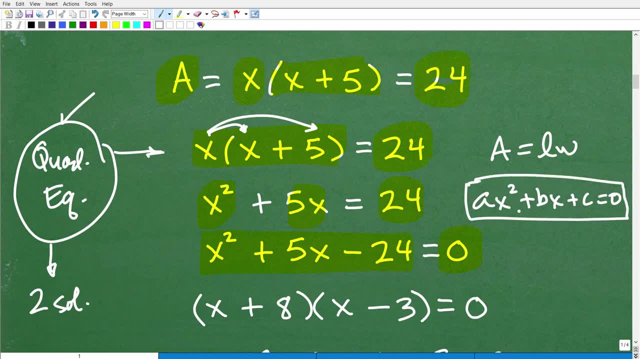 So we need to oftentimes have an equation, A quadratic equation, in standard form, Because if we can't solve this equation easily- And I'm talking about how, the way I solved it- Then we're going to have to use what You're going to have to use: a quadratic formula. 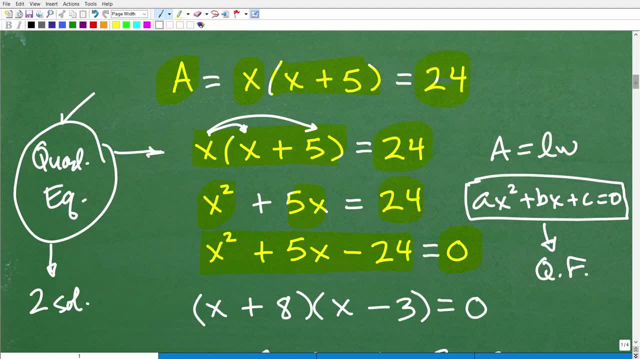 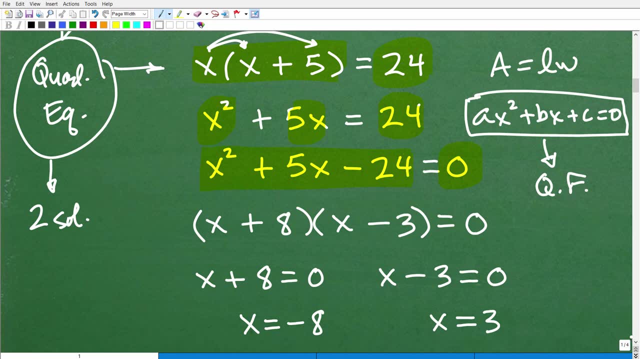 So I'm kind of giving you a little additional bonus material about quadratic equations. If you're struggling with quadratic equations, I would definitely suggest that you check out, like my, Algebra 1 course, Algebra 1, Algebra 2.. Whatever level that you're at, 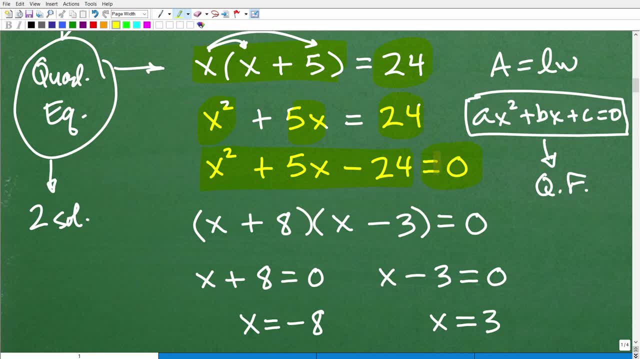 Okay, So here we have x squared plus 5x minus 24 is equal to 0.. So what's the first step, The first thing you want to do? Well, we have a quadratic trinomial. You want to attempt to factor this: 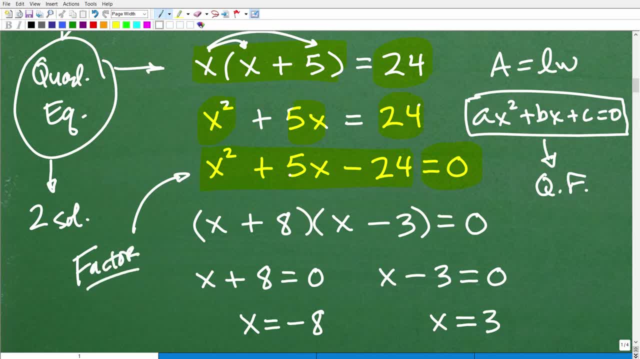 Okay, We always want to factor when we can, But sometimes we can't factor. And when we can't factor we're going to have to go to the quadratic formula. But in this case I made this problem nice and easy. This quadratic trinomial factors as x plus 8 times x minus 3.. 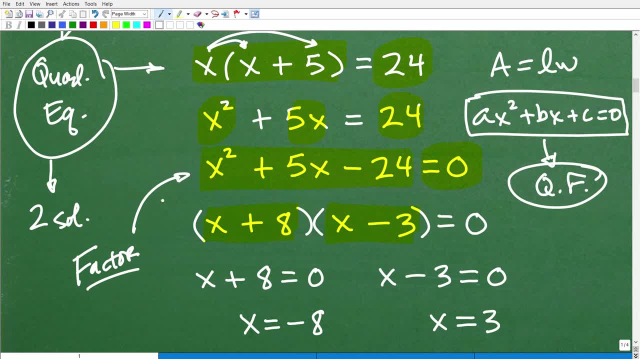 Now, can you factor this? Okay, Do you have the skills to factor this? And here is the answer: Okay, If you don't know how to factor this, would be an algebra emergency. Okay, So in other words, sirens going off everything else. 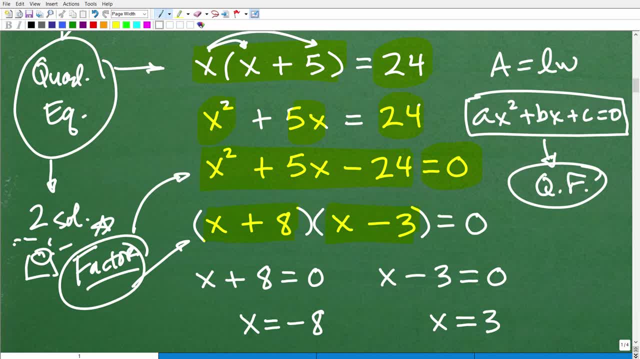 You absolutely must be a master at factoring to be successful in algebra. So again, go back and just make note of what you know and don't know and review this. Okay, Again, you know I'm kind of being redundant. 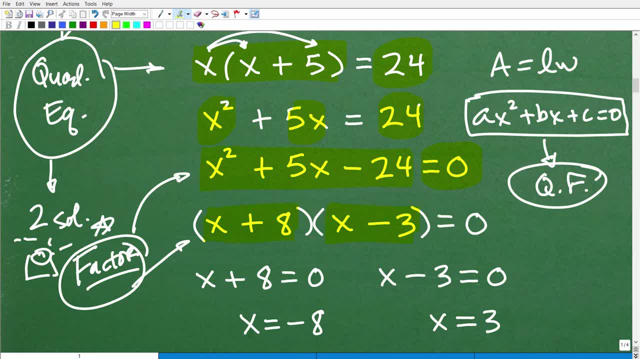 But if you're taking any sort of algebra course, factoring quadratic equations, absolutely, they're just everywhere. Okay, You can't pass algebra without knowing this stuff, Okay, So here we have x plus 8 times x minus 3.. 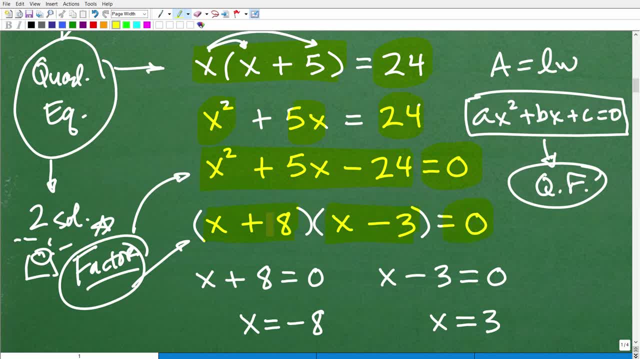 This is equal to 0. So we're going to set each of these factors equal to 0. So it's x plus 8 is equal to 0 and x minus 3 is equal to 0. Then we're going to go ahead and solve the respective equation. 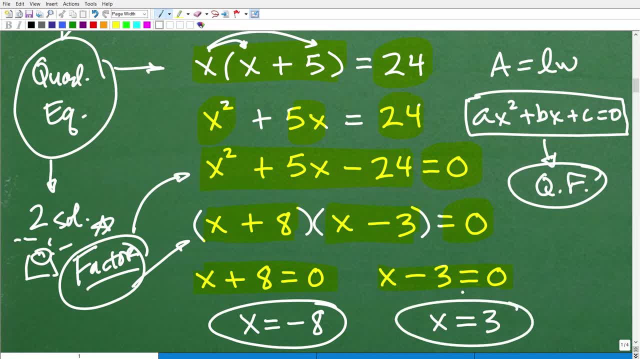 So here we have: x is equal to negative 8.. In this equation we have: x is equal to 3.. So these are our two solutions, But we need to think about this for a second Like. well, which answer do I use? 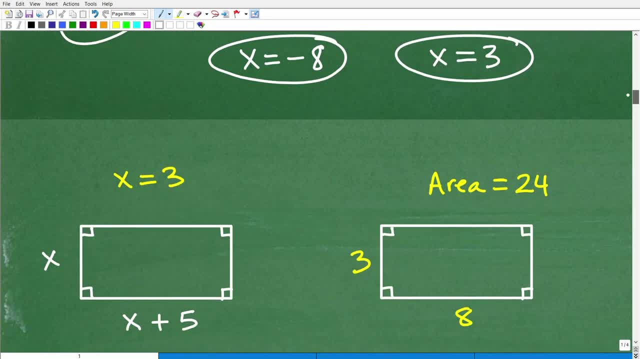 Well, remember, x represents a side, It represents distance, right, So are we going to have a negative distance? We're like, no, that's not going to make sense. So we're going to throw that negative out, that negative solution out. 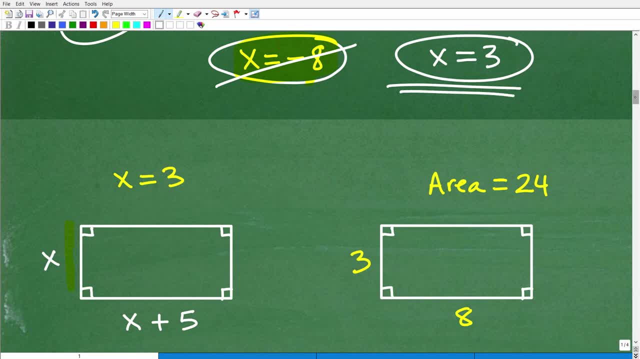 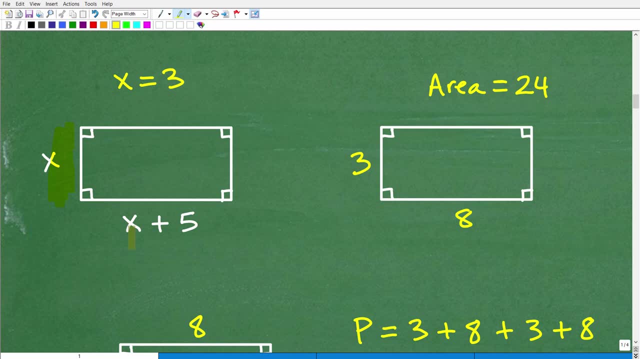 And we'll keep the positive solution. So x is equal to 3.. Okay, So that's how we solve for x. So that means this side of this rectangle would be 3. And this side would be what? 3 plus 5 or 8.. 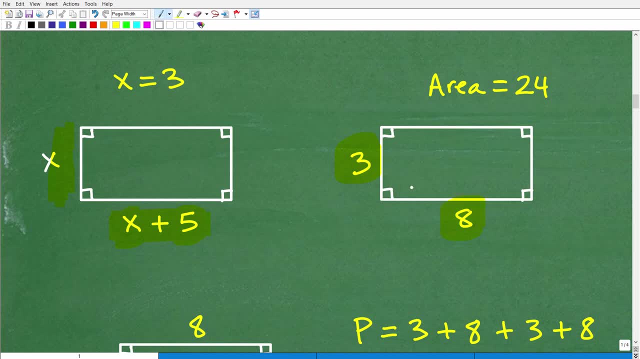 Okay, So we have 3 and 8.. Well, let's just check this here. If I wanted to find the area of this rectangle, it would be what, The length times the width, or 8 times 3.. And that, in fact, checks out as 24, which is what we were told. 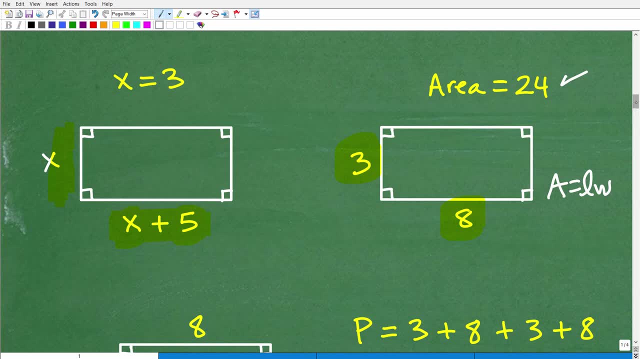 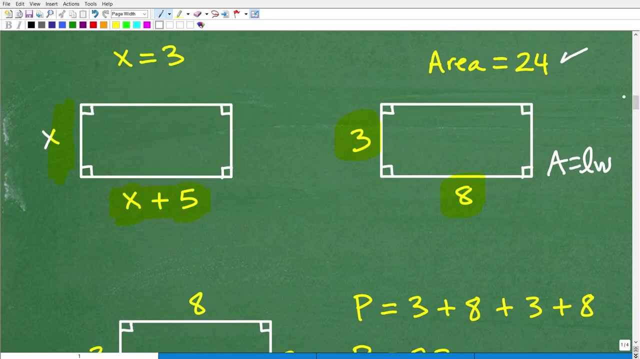 Okay, So this is good, And right now, we need to now get into the perimeter. So what is the perimeter Actually? let me show you right here What is the perimeter of a rectangle, or a perimeter of anything? Well, it's the distance. 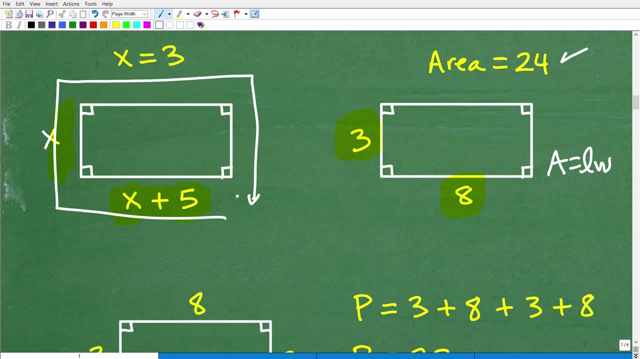 The distance around the entire figure. In this case we're dealing with a rectangle, So we're going to have to add up this side, this side, this side and this side. So you need to know that a rectangle, opposite sides are congruent, ie the same.